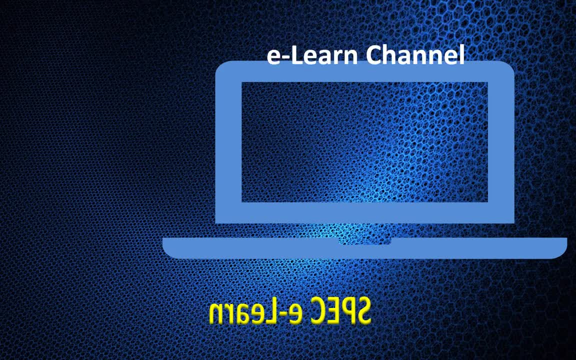 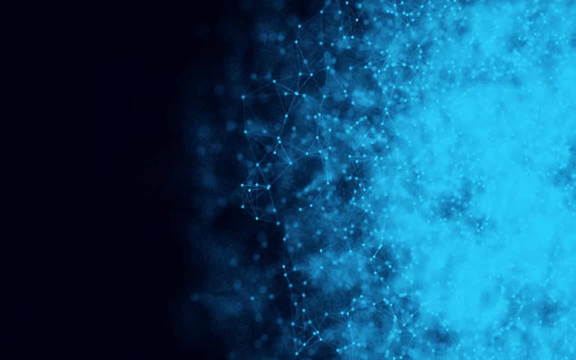 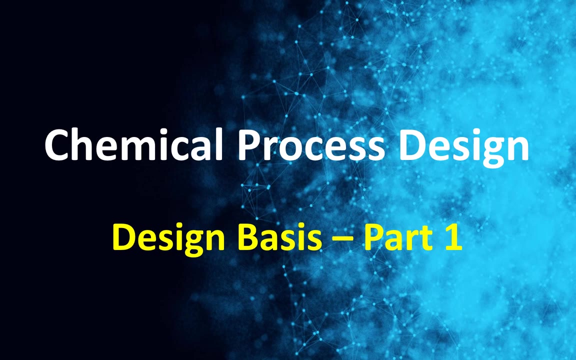 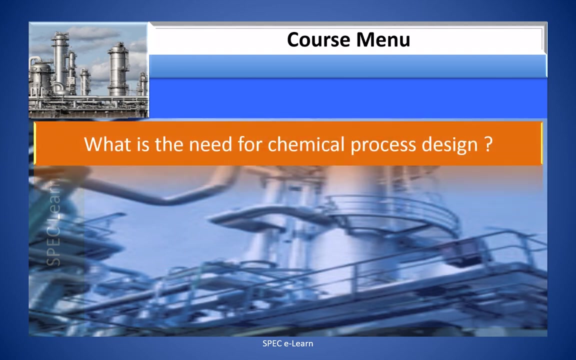 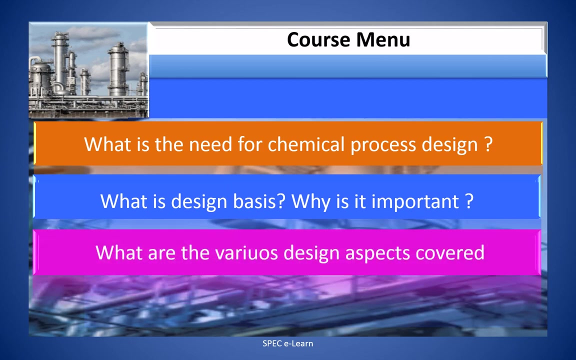 Hello everyone, welcome to SPECT eLearn, the online learning channel dedicated to chemical engineers. In this video course, you will learn What is the need for chemical process design, What is the design basis, Why is it important? What are the various design aspects covered? 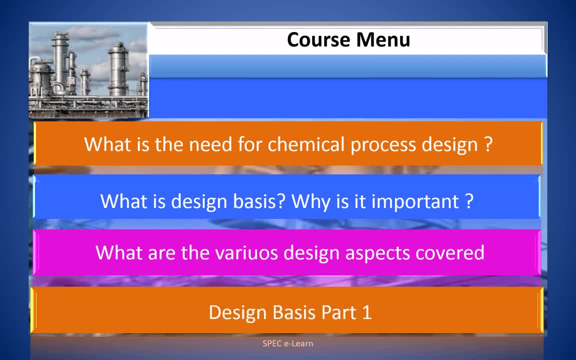 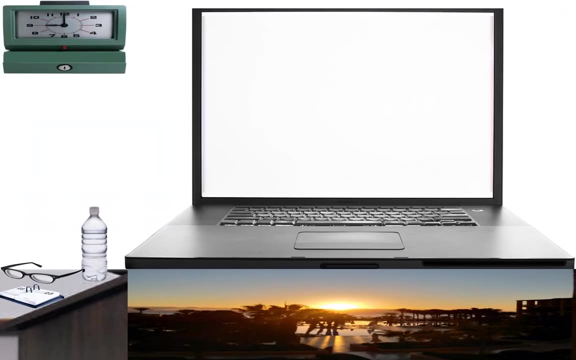 Design basis, part 1. Please subscribe to the channel. By subscribing, you will motivate us to produce knowledgeable video content for you. So subscribe now, before you forget. A chemical process plant is a production asset designed and built for conversion of raw material into finished products. 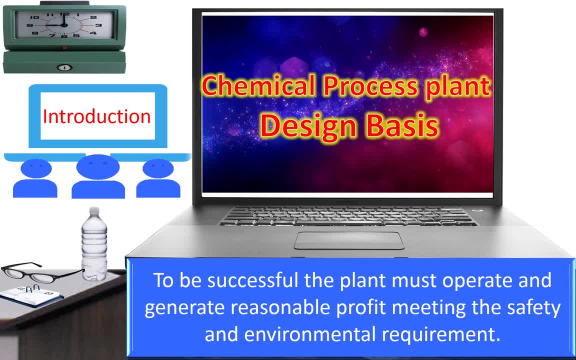 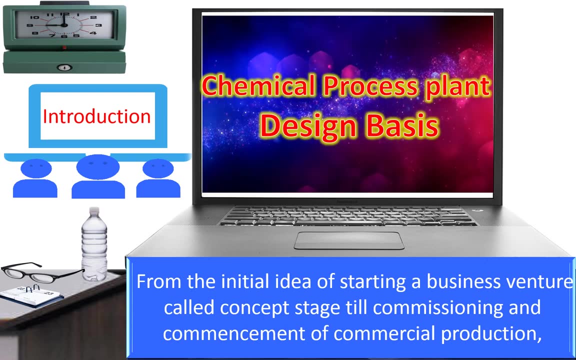 To be successful, the plant must operate and generate reasonable profit, meeting the safety and environmental requirement. From the initial idea of starting a business venture, called concept stage, till commissioning and commencement of commercial production, the setting up of a chemical process plant goes through a series of stages. 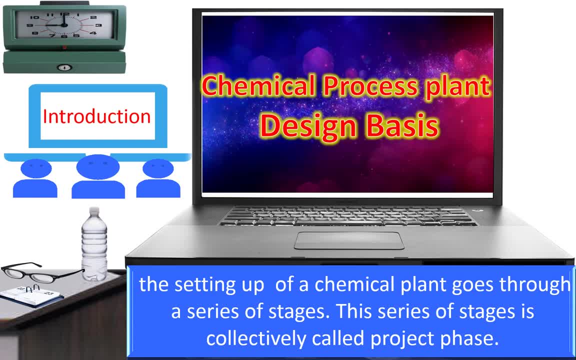 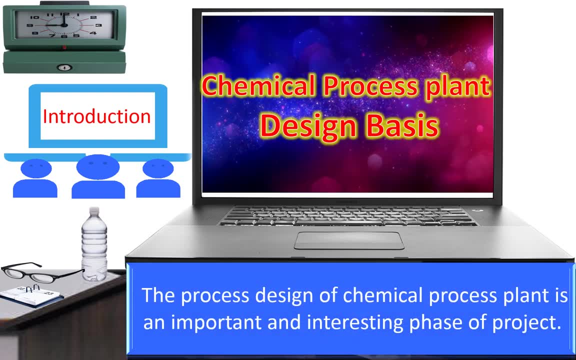 This series of stages is collectively called project phase. The process design of a chemical process plant is an important and interesting phase of the project. It's a very complex and complex process. The design process is a very complex process. It's a very complex process. 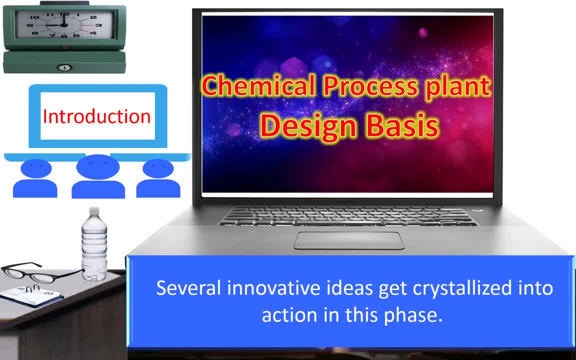 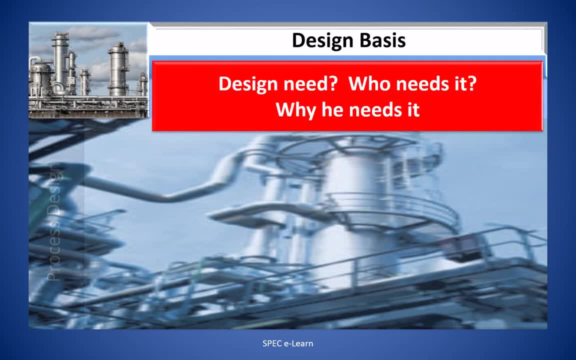 There are several innovative ideas that get crystallized into action in this phase. The design process is a very complex process. The design process is a very complex process. It's a very complex process. Design needs Who needs it And why he needs it. 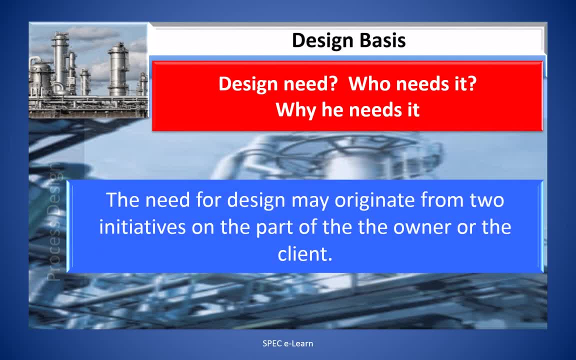 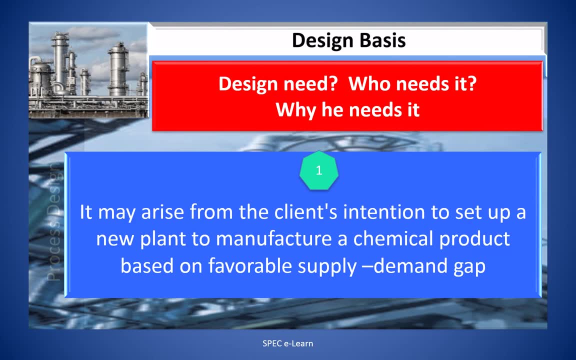 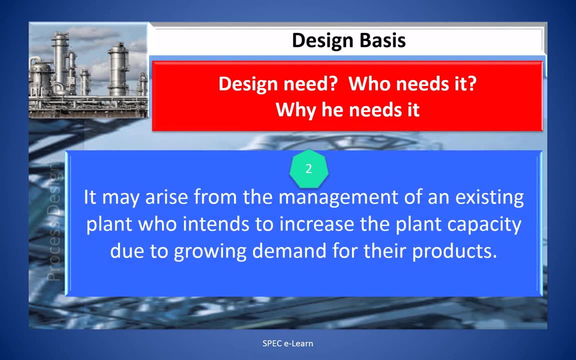 The need for design may originate from two initiatives on the part of the owner or the client. One: it may arise from the client's intention to set up a new plant to manufacture a chemical product based on favorable supply-demand gap. Two: it may arise from the management of an existing plant. 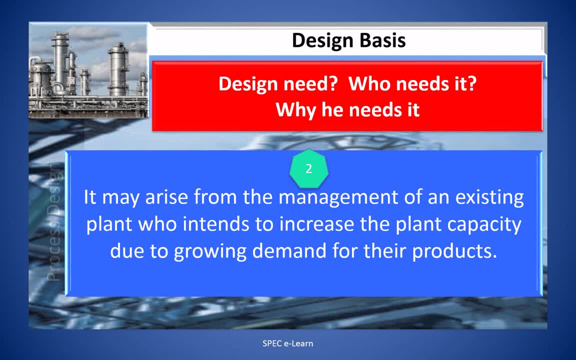 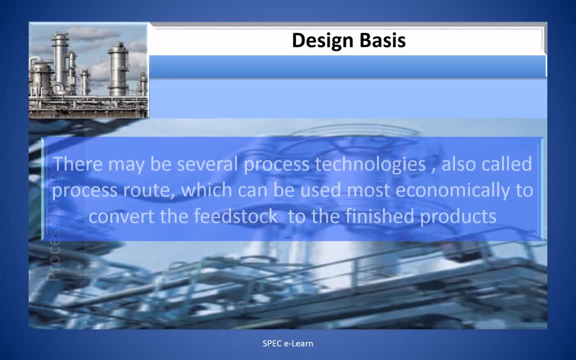 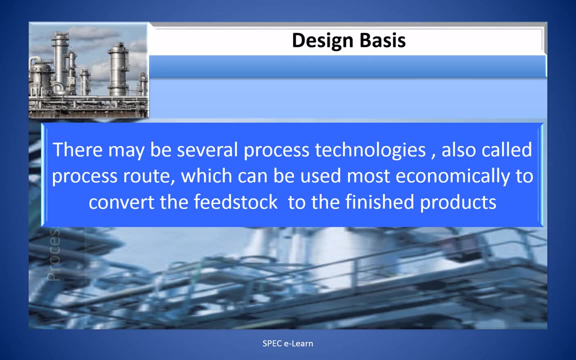 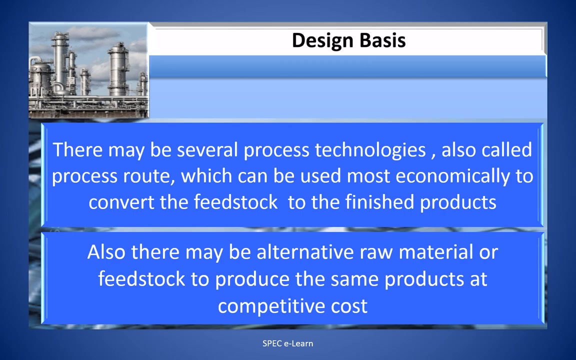 who intends to increase the plant capacity due to growing demand for their products. There may be several process technologies, also called process route, which can be used most economically to convert the field stock to the finished products. Also, there may be alternative raw material or feedstock to produce the same product at. 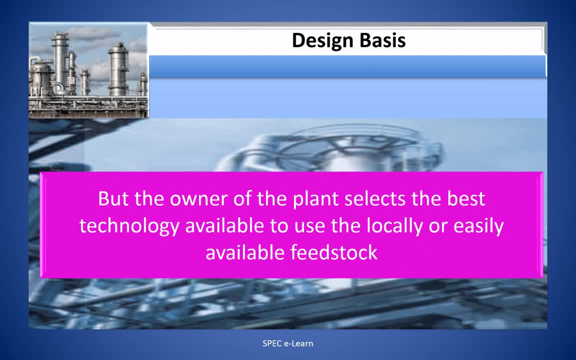 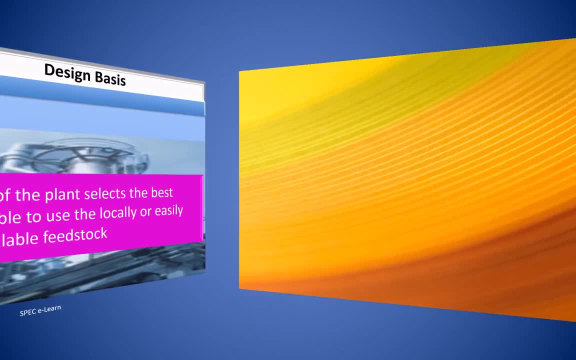 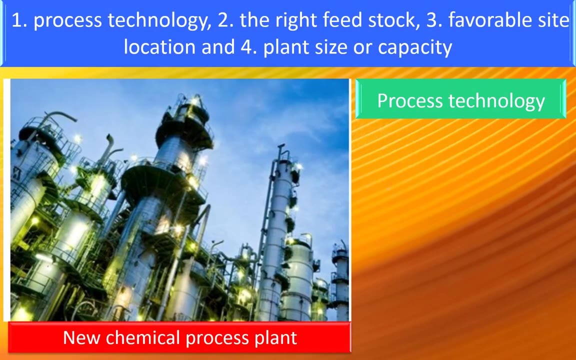 competitive cost. But the owner of the plant selects the best technology available to use a locally or easily available feedstock. So the key to success of the venture lies in the selection of: one: process technology. two, the right feedstock. three, favorable site location. 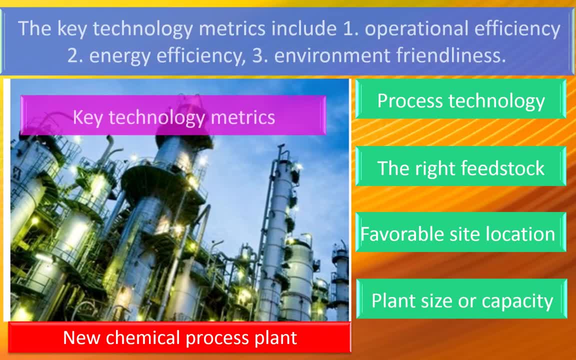 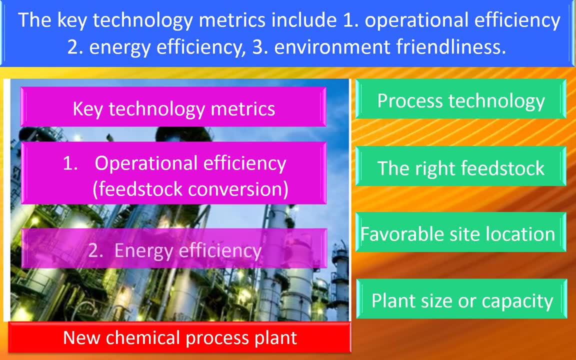 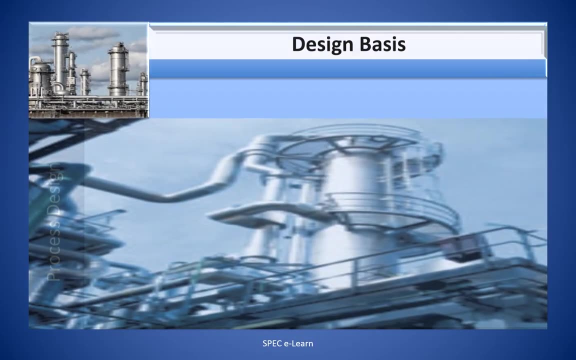 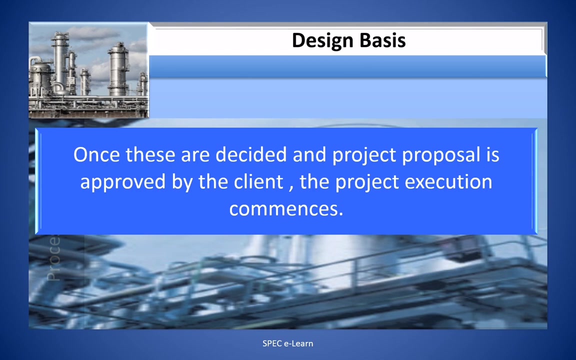 four: plant size or capacity. The key technology metrics include operational efficiency, energy efficiency and environmental friendliness. Once these are decided and the project proposal is approved by the client, the project execution commences. The project goes through three phases of execution. 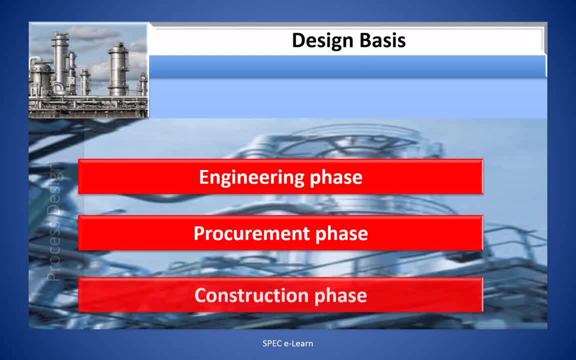 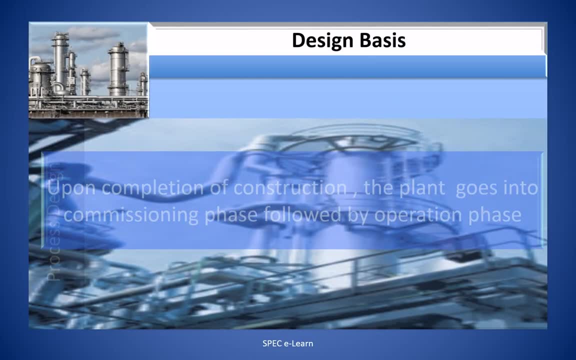 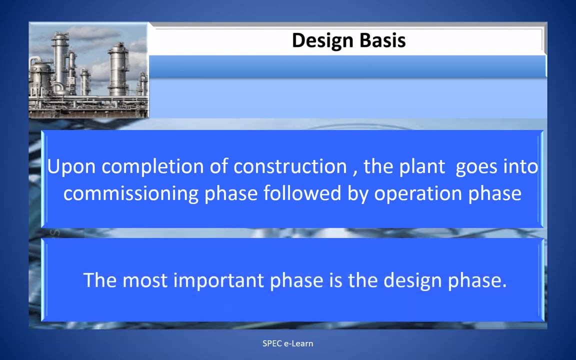 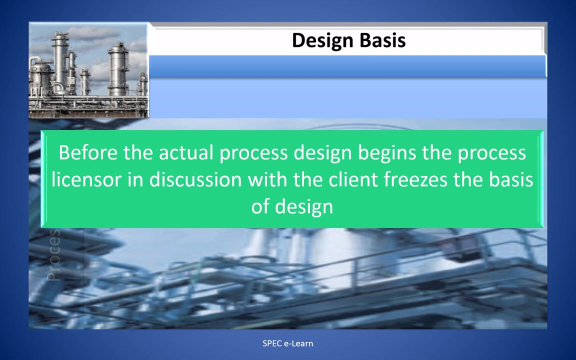 engineering phase, procurement phase and construction phase. Upon completion of construction, the plant goes into commissioning phase, followed by operational phase. The most important phase is the design phase. Before the actual process design begins, the process licensor, in discussion with the client, freezes the basis of design. This is an important document. 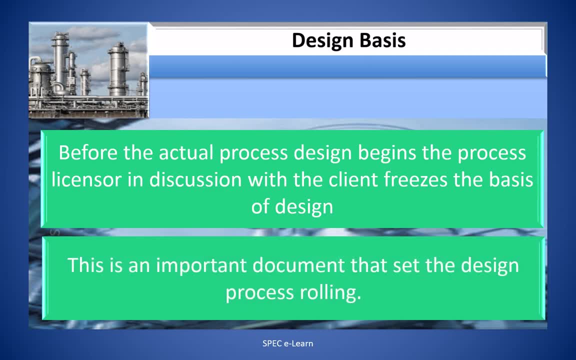 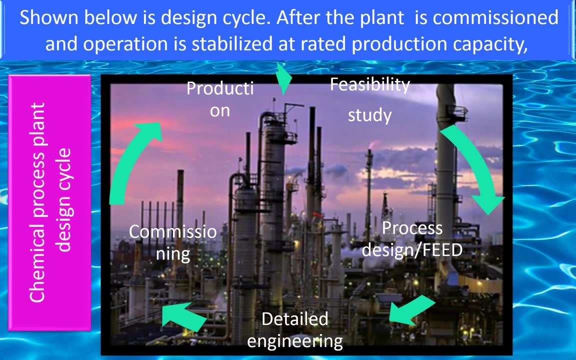 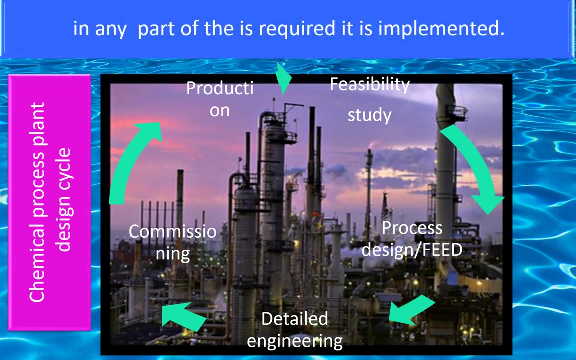 that sets the design process rolling. Shown below is the design cycle After the plant is commissioned and operation is stabilized at rated production capacity. any design discrepancy against design basis is analyzed and if modification in design in any part of the plant is required, it is implemented. The cycle repeats till 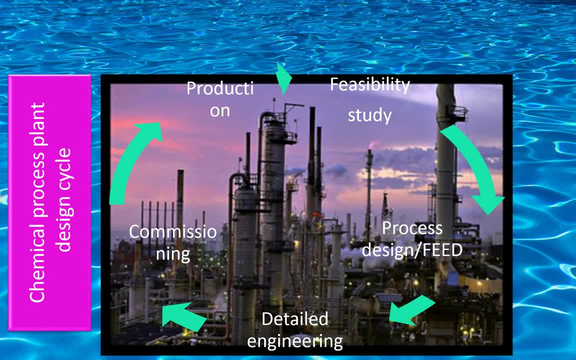 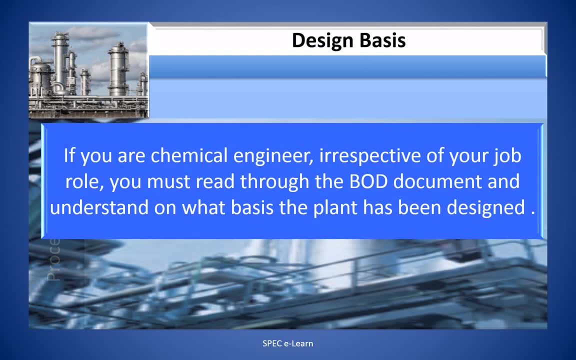 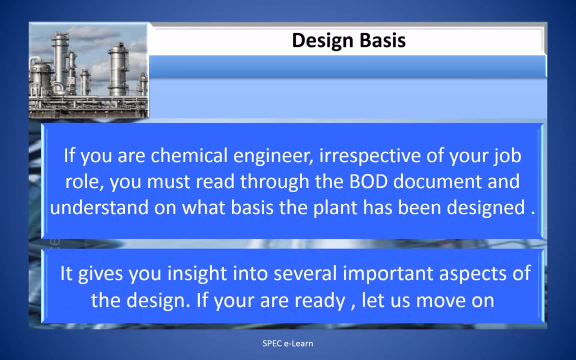 the plant operates as per the original design basis. If you are a chemical engineer, in respect of your job role, you must read through the BOD document and understand on what bases the plant has been designed. It gives you an insight into several important aspects of the design. 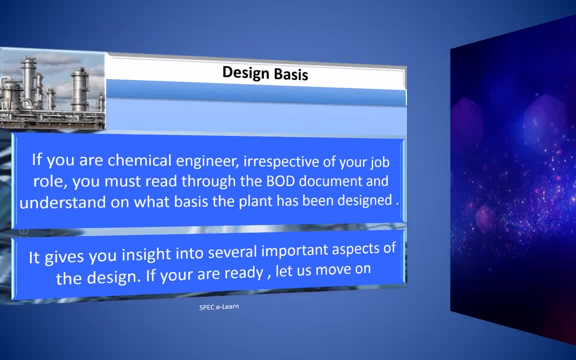 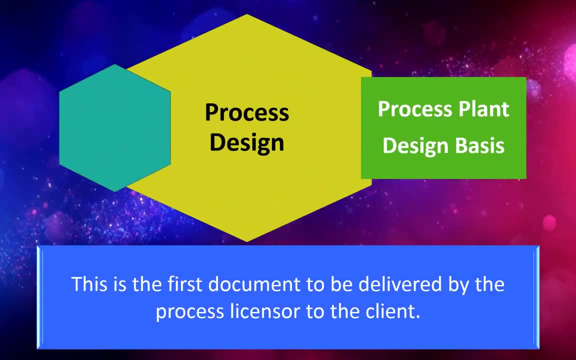 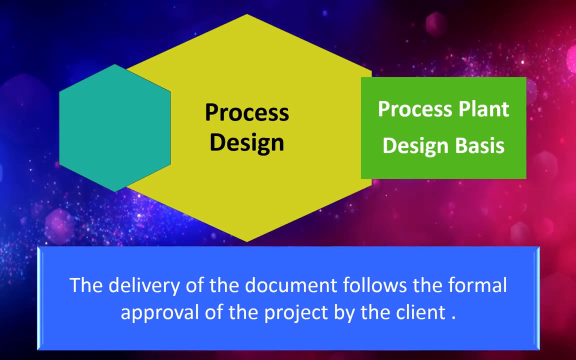 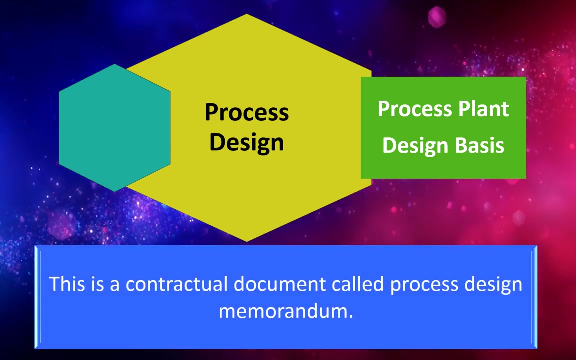 If you are ready, let us move on. Process Plan- Design Basis. This is the first document to be delivered by the process licensor to the client. The delivery of the document follows the formal approval of the project by the client. This is a contractual document called Process Design Memorandum. 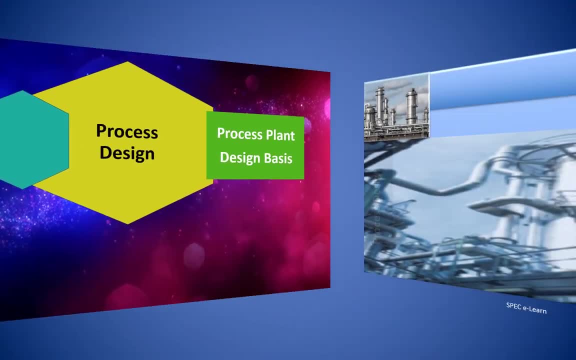 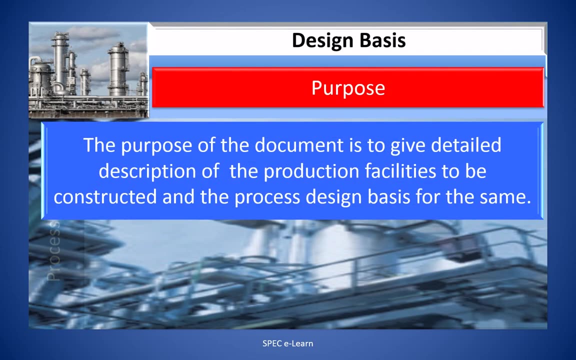 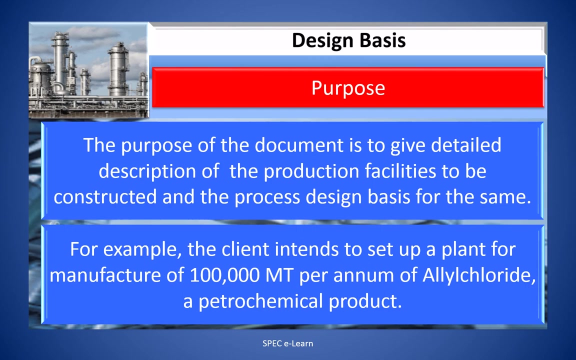 The purpose of this document is to give a detailed description of the production facilities to be constructed and the process design basis for the same. For example, the client intends to set up a plant for manufacture of 100,000 mT per annum of Allyl Chloride, a petrochemical product. 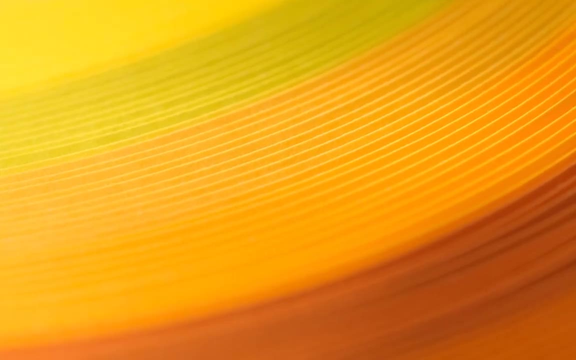 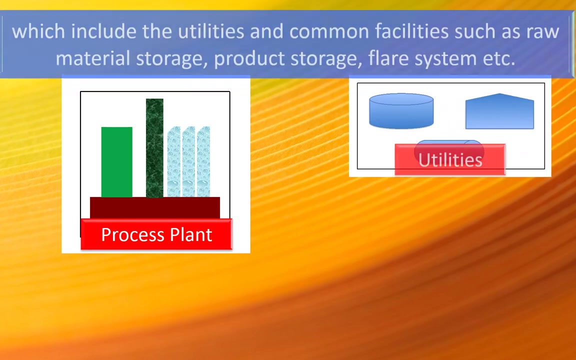 The plant will have the following requirements. The plant will have the following requirements. We have the main process plan to produce Allyl Chloride and support facilities, which include the utilities and common facilities such as raw materials storage, product storage, flyer system, etc. 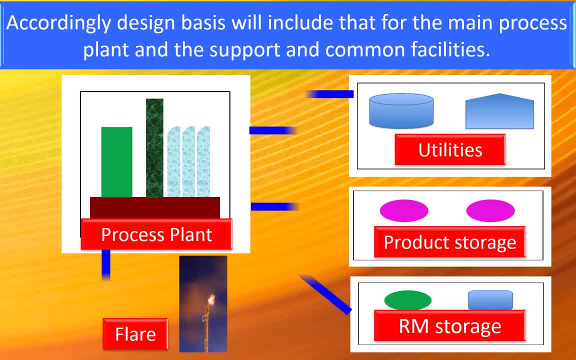 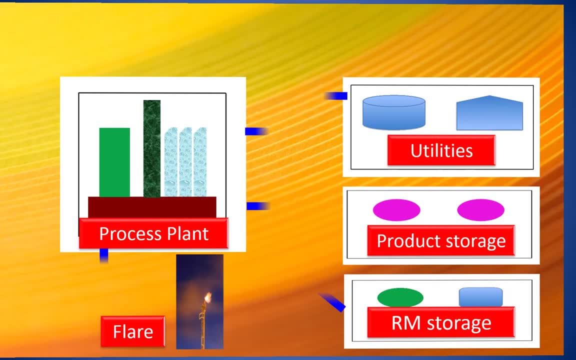 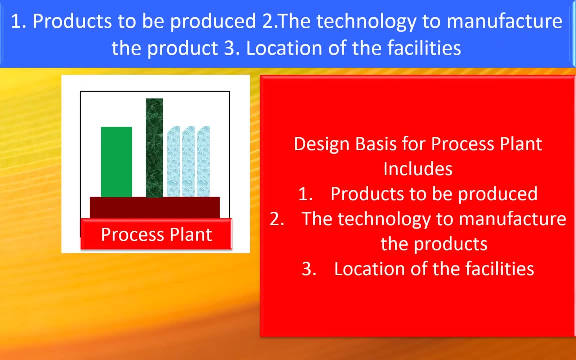 Accordingly, the design basis will include those for the main process plan and the support facilities. The design basis for the process plan includes the following One: The products to be produced. 2. The technology to manufacture the product. 3. The location of the facilities. 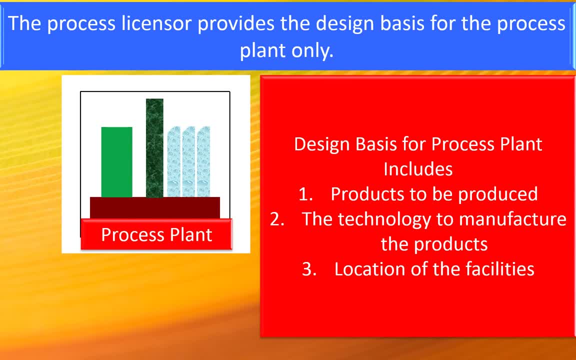 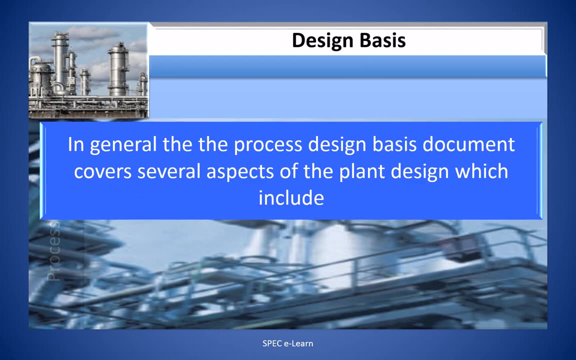 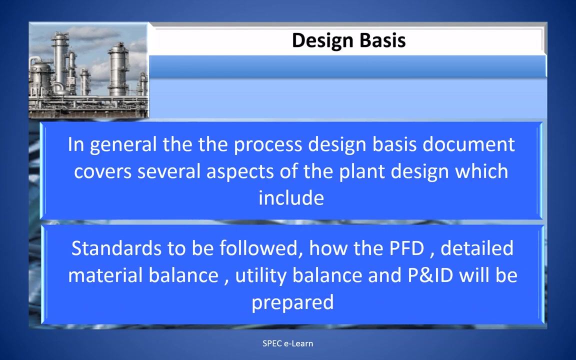 The process licensor provides the design basis for the process plant only. For the support facilities, the design basis is developed and provided by the detailed engineering consultant. In general, the process design basis document covers several aspects of the plant design, which include standards to be followed how the PFD, detailed, material balance, utility balance. 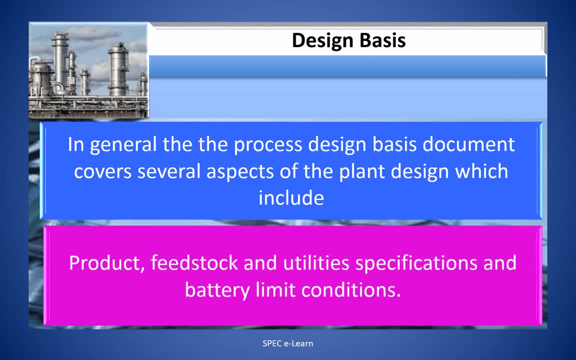 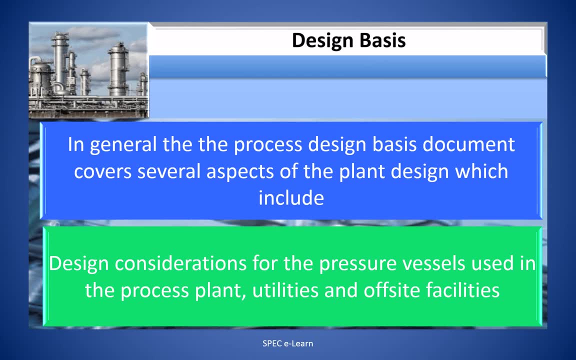 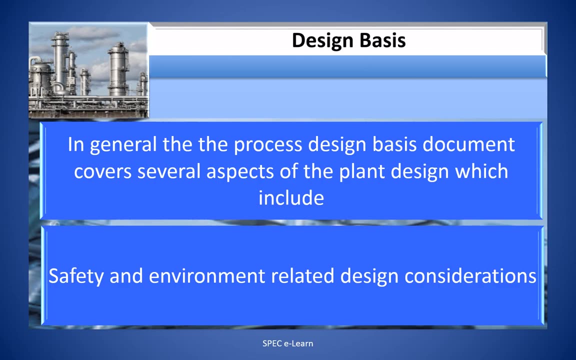 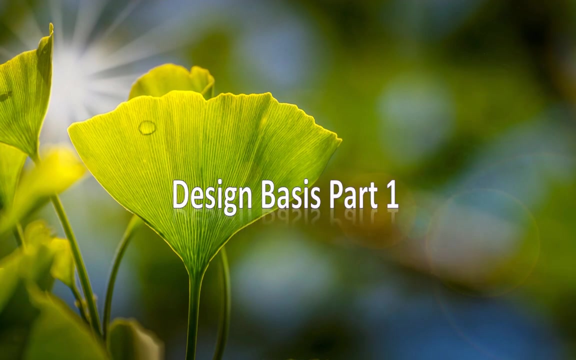 and P&AD will be prepared. product feedstock and utility specifications and bed limit conditions. design consideration for the pressure vessels used in the process, plant utilities and off-site facilities. safety and environmental related design considerations. Design basis- part 1.. In part 1, you will get an insight into some of the design aspects mentioned above. 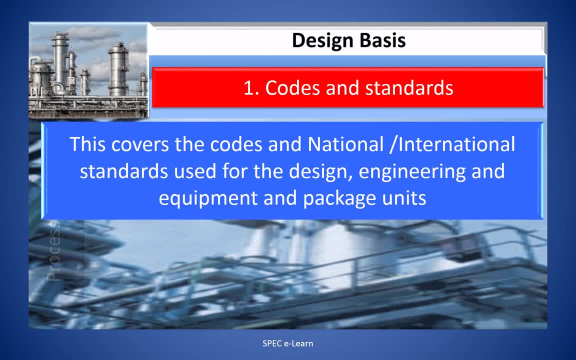 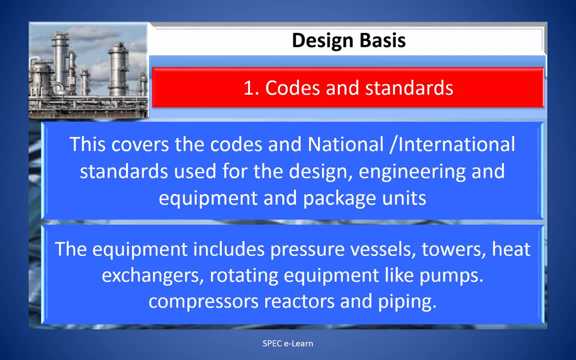 1. Codes and Standards. This covers the codes and national and international standards used for the design, engineering equipment and package units. Equipments include pressure vessels, towers, heat exchangers, rotating equipment like pumps and compressors, reactors and piping. 2. There are several codes and standards covering all of these. 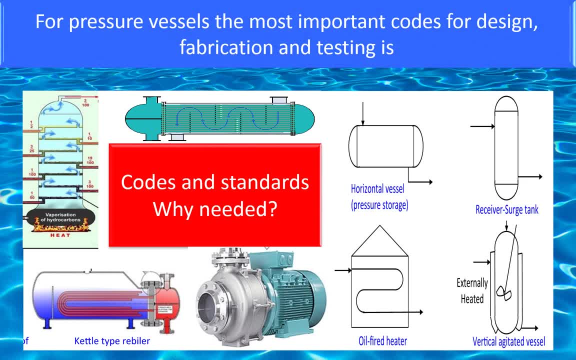 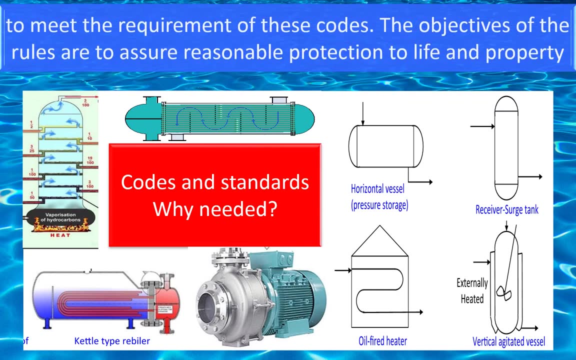 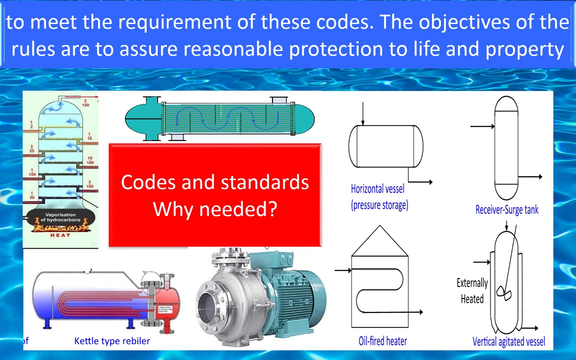 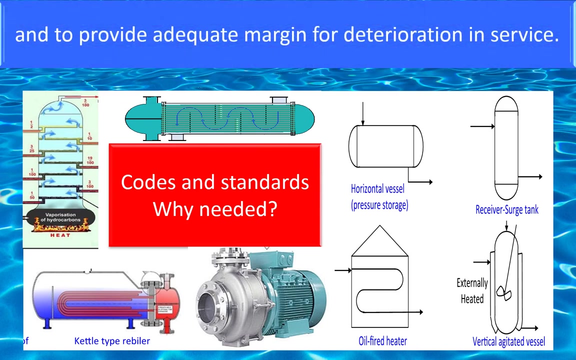 For Pressure Vessels. the most important code for design, construction and testing is American Society of Mechanical Engineers boiler and pressure vessel code. The pressure containing components called pressure pots may be required by law to meet the requirements of these codes. The objectives of the rules are to assure reasonable protection to life and property and to provide adequate margin for deterioration in service. 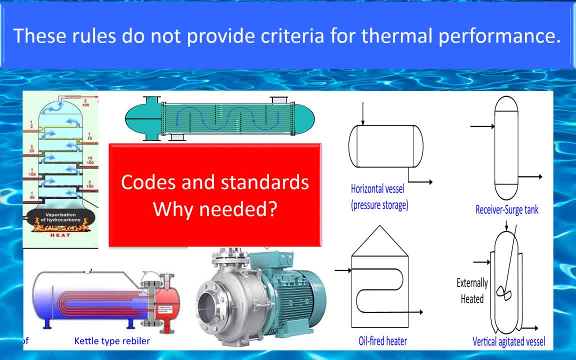 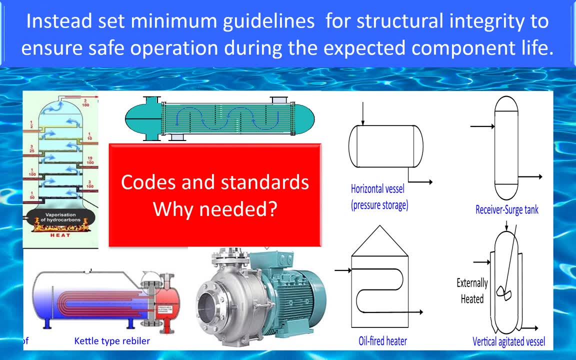 These rules do not provide criteria for thermal performance. Instead set minimum guidelines for structural integrity to ensure safe operation during the expected equipment life. Following the codes will ensure development of safe pressure welder design. The same is the case with other process equipment such as heat exchangers, reactors, rotating equipment, storage tank, etc. where codes such as API and TEMA are used. 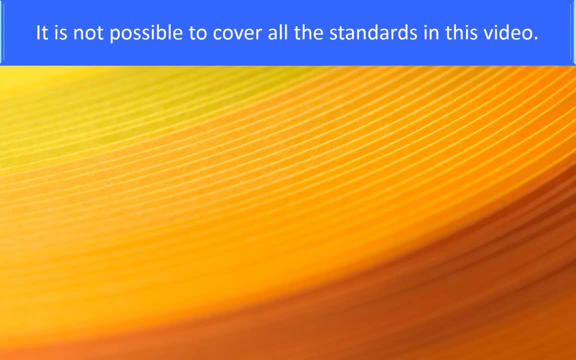 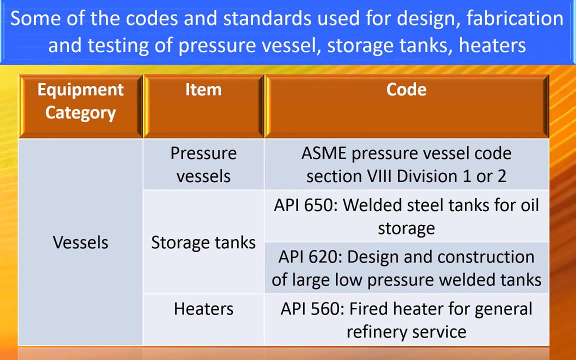 It is not possible to cover all the standards in this video, But some of the codes and standards used for design, fabrication and testing of pressure vessel storage tank heaters, heat exchangers, rotating equipment, wiping are given in the table below. 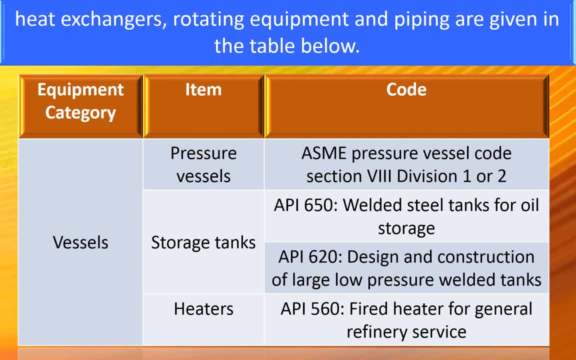 Pressure Vessels- ASMA Pressure Vessel Code Section 8, Division 1 or 2. Storage Tanks- API 650- for Welded Steel. Tanks for Oil Storage- API 620- Design and Construction of Large and Low Pressure Tanks. Heaters- API 560- Fad Heater for General Refinery Service. 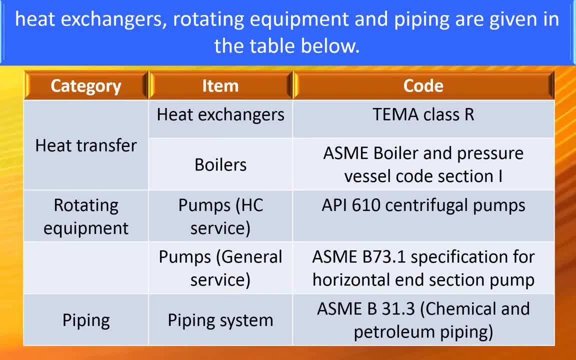 Heat Exchangers. TEMA: Class R Boiler- ASME. Boiler and Pressure Vessel. Code Section 1: Pumps for Hydrocarbon Service- API 610- Centrifugal Pumps. Pumps for General Service- ASME B73.1. Specification for Horoscope INFUNCESS. 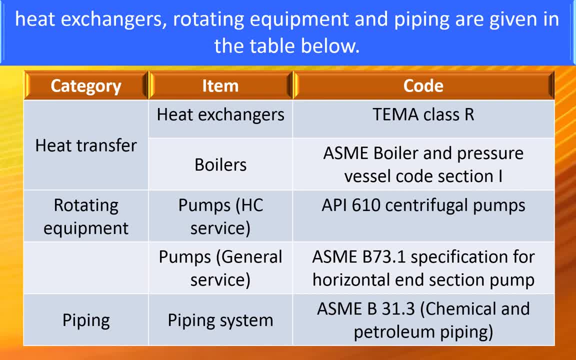 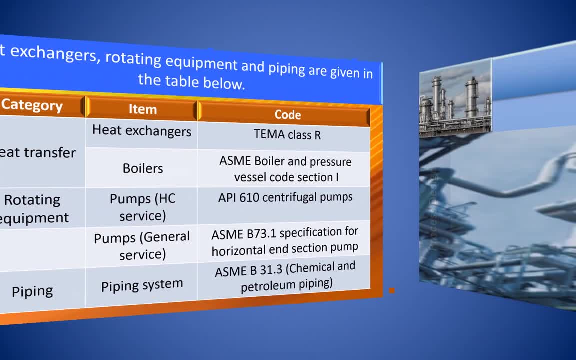 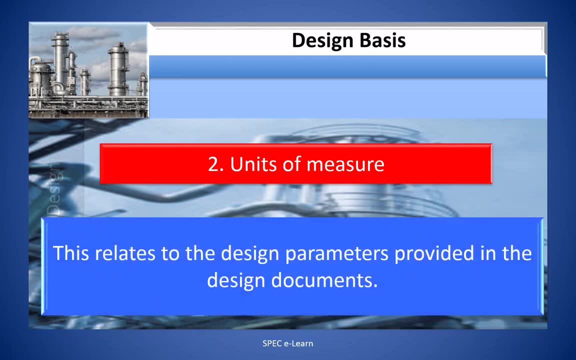 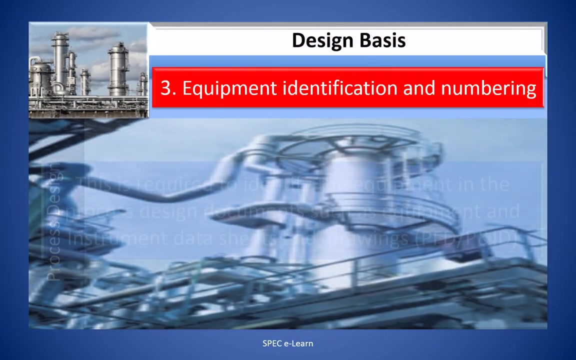 ASME B71.2 Specification for Horizontal N Section Pump. Types of Inable Pumps. Types of Disпарced Pumps. 2. Unit Submeasure. Types of Imples. 3. Equipment Identification and Numbering. This is required to identify the equipment. 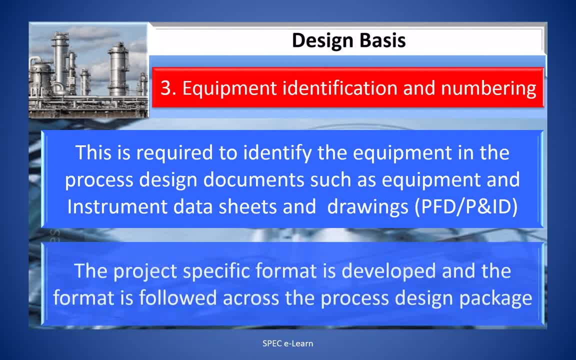 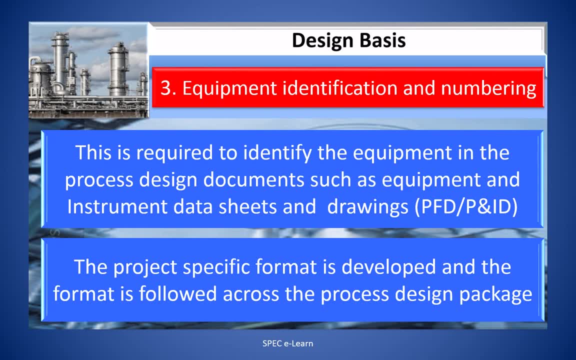 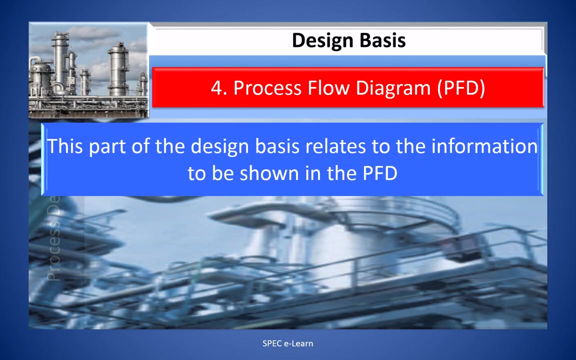 in the process design documents, such as equipment and instrument data sheets and drawings like PFD and P&ID, The project specific format is developed and the format is followed across the process design package. 4. Process Flow Diagram. This part of the design basis relates to the information. 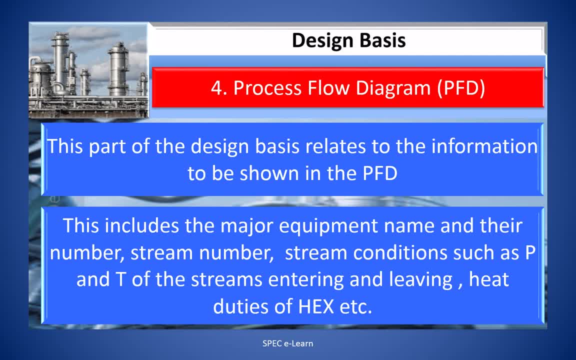 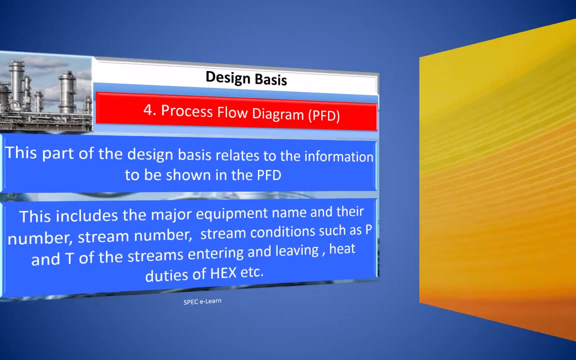 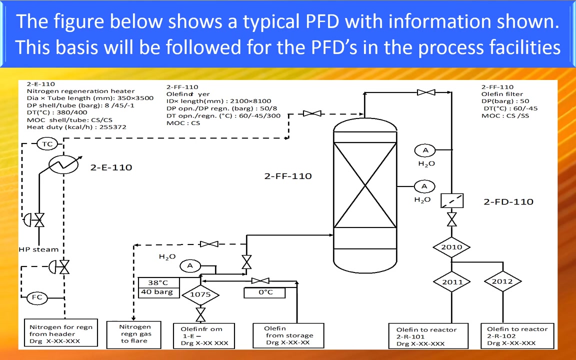 to be shown in the PFD. This includes the major equipment name and day number, stream number, stream conditions such as pressure and temperature of the streams entering and leaving, heat duties of heat exchangers, etc. The figure below shows a typical PFD with information shown. This base will be followed. 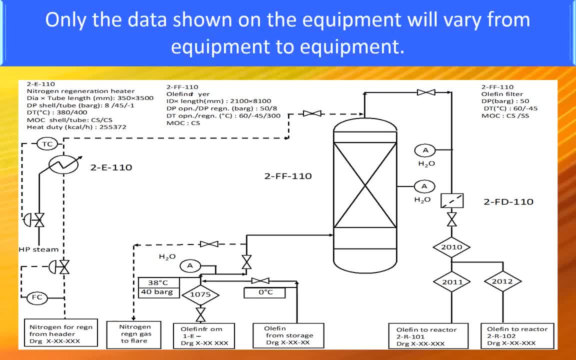 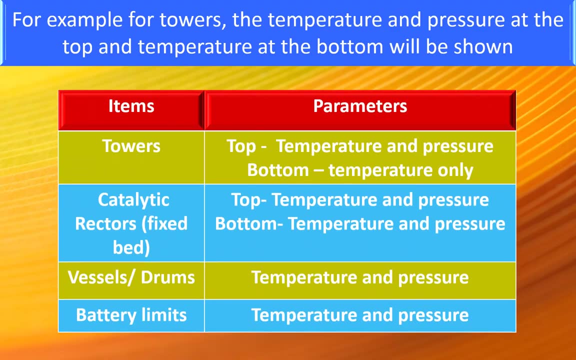 for the PFDs in the process facilities Only. the data shown on the equipment vary from equipment to equipment. This is because functionally each equipment is different. For example, for towers, the temperature and pressure at the top and temperature at the bottom will. 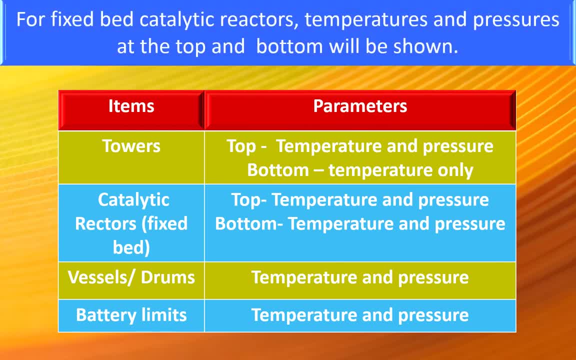 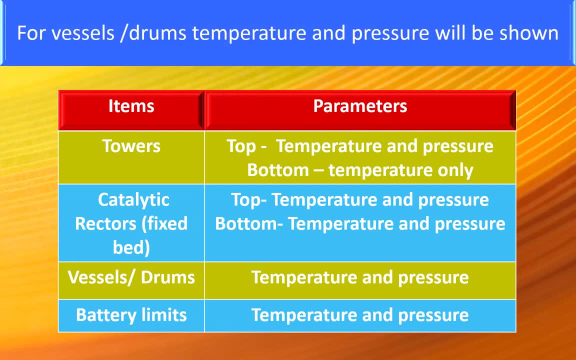 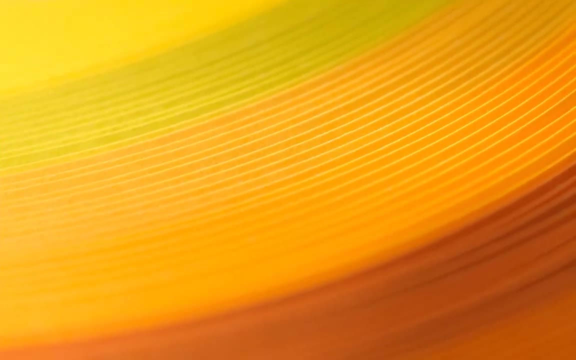 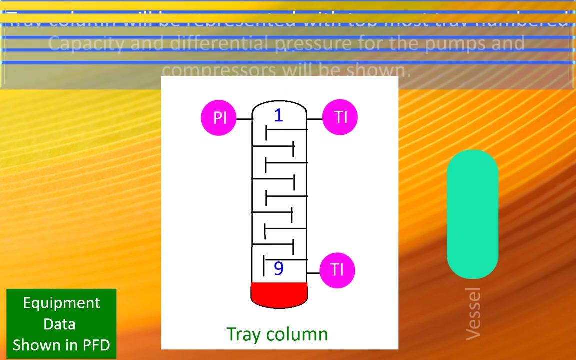 be shown. For fixed batteries, the temperature and pressure at the top and temperature at the bottom will be shown. For the column will be represented with the topmost tray numbered 1.. Capacity and differential pressure for the pumps and compressors will be shown. 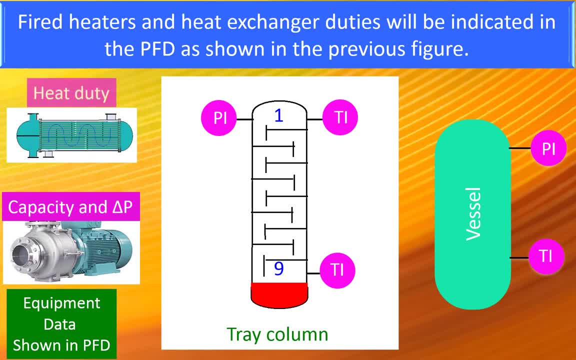 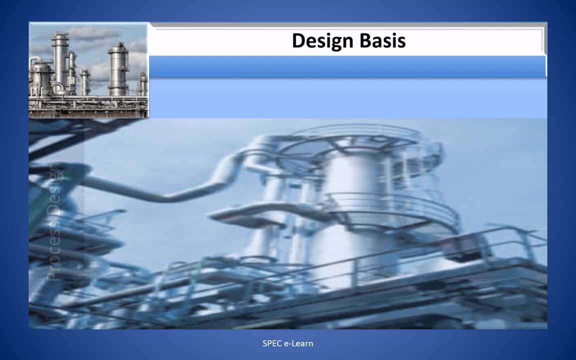 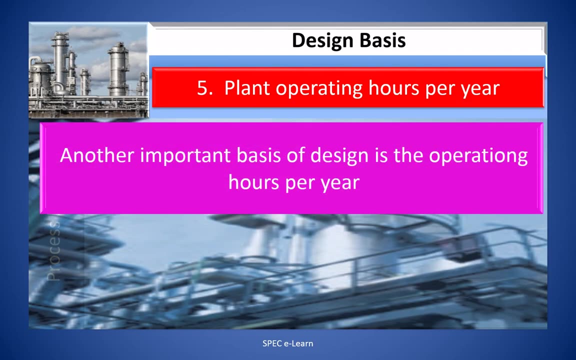 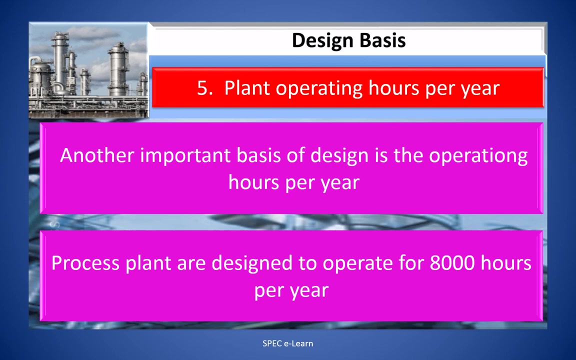 Fired heaters and heat exchangers, duties will be shown. Duties will be indicated in the PFD as shown in the previous figure 5.. Plant operating hours per year. Another important basis of design is the operating hours per year. Process plants are designed to operate for 8000 hours per year. 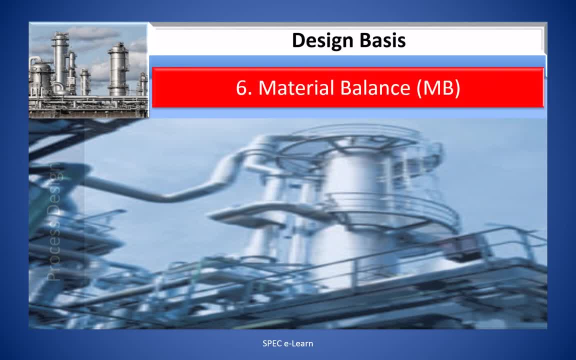 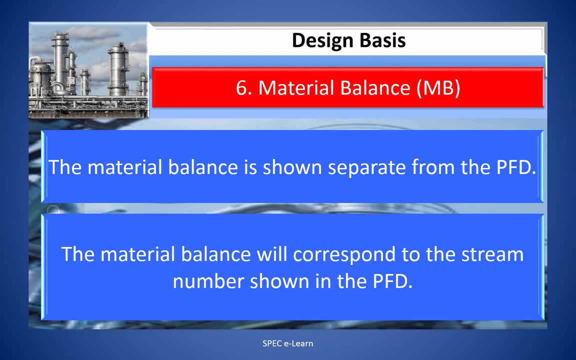 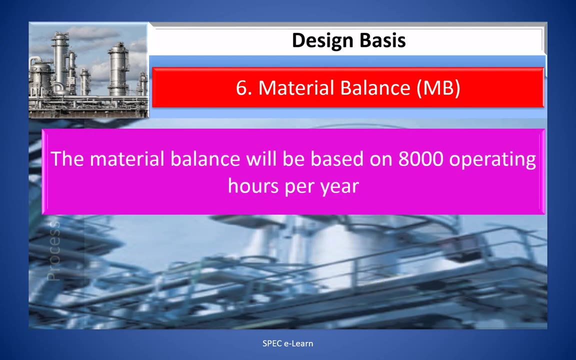 6. Material balance. The material balance is shown separate from the PFD. Material balance will correspond to the stream number shown in the PFD. The material balance will be based on 8000 operating hours per year If the annual production capacity is 100000 metric tons per year. the hourly 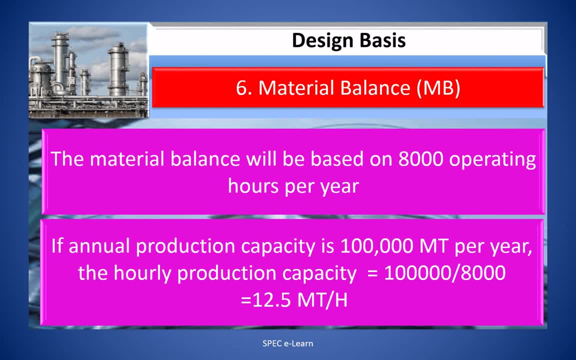 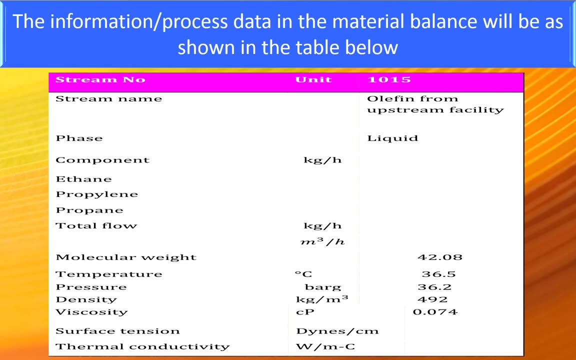 production capacity is calculated as 100000 divided by 8000, which is equal to 12.5 metric tons per hour. The information or process data in the material balance will be as shown in the table below. The process information include the stream number and the unit submission Under the 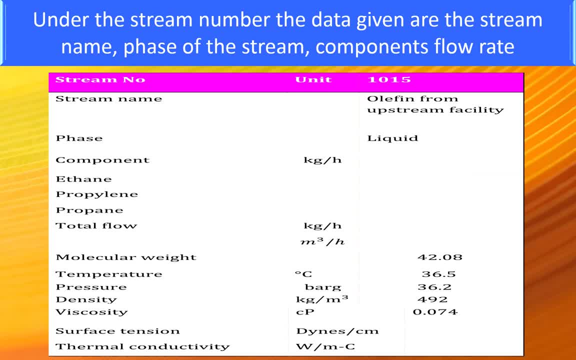 stream number. the data given are the steam name, phase of the stream, components, flow rate, molecular weight and the temperature. The process information will be as shown in the table below. The process information includes the floor rate, temperature, temperature and thermodynamic. 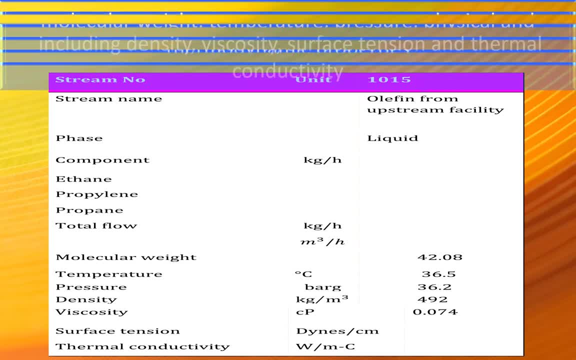 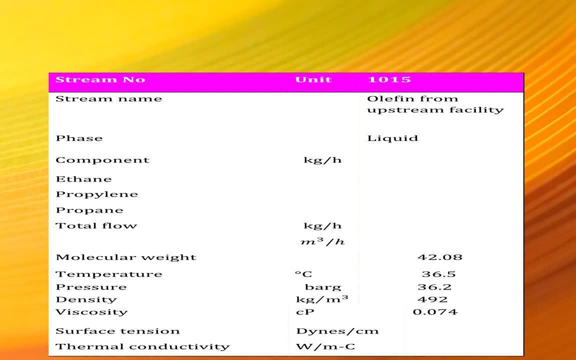 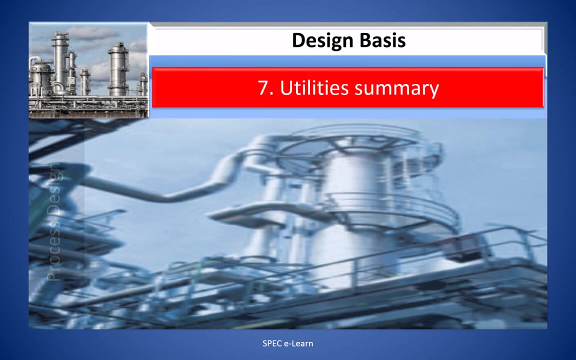 properties, including density, viscosity, core to form surface tension and thermal conductivity. In case the are two-phase governments, floor rate of both liquid and vapor would be shown 7. Utility summary and fail balance include the following: steam and condensate, cooling water, demineralized water, nitrogen.